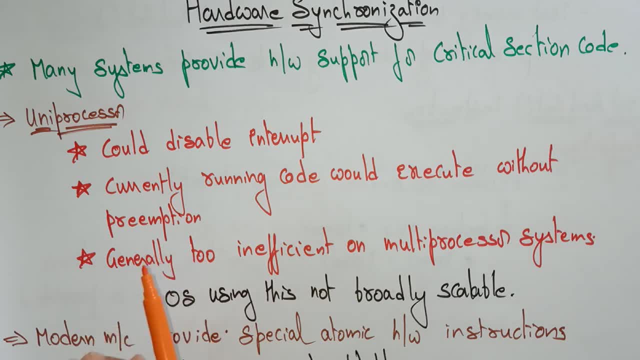 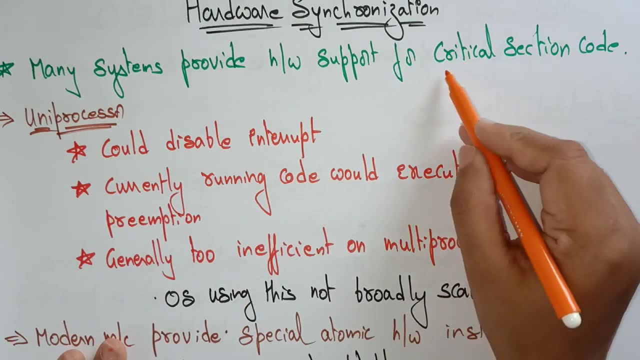 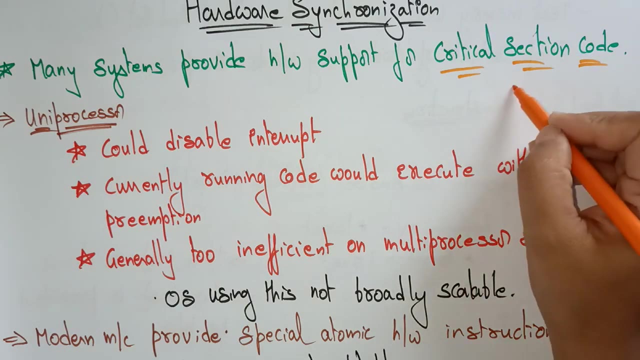 then only our systems will work efficiently. So let's have a look on this hardware synchronization. Many systems provides a hardware support for critical section code. Let's talk about this critical section code. So you know that the critical section code, that means it is a code where whenever one process 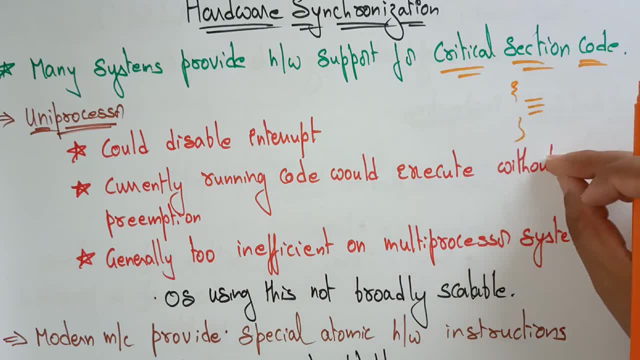 is executing in the critical section code, no other processor will enter into that stage. After the completion of this section code, another processor will end. Suppose P1 is executing. P2 has to wait until P1 is completed in the critical section code. Whenever P1 is completed, it comes. 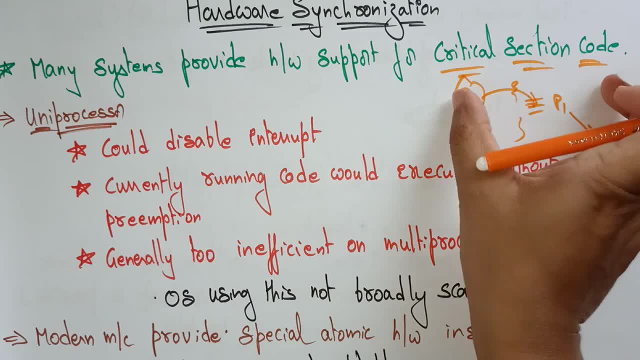 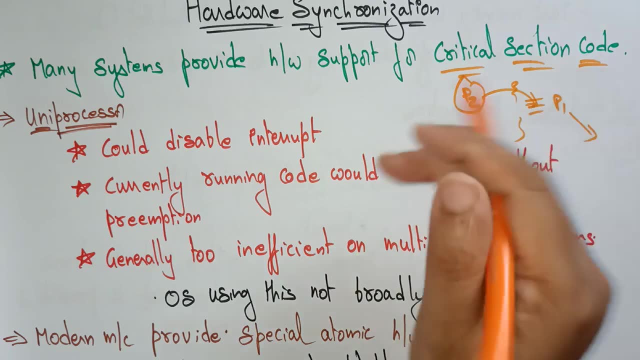 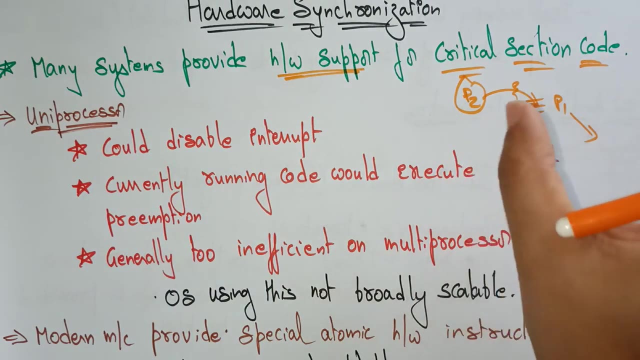 out and P2 will enter into the critical section code. So this is a critical section code. So we know that. so to work like this properly, we requires the hardware support also. Many system provide hardware support for this critical section code. So let's first have a look on what is this hardware support? I said many system provides. 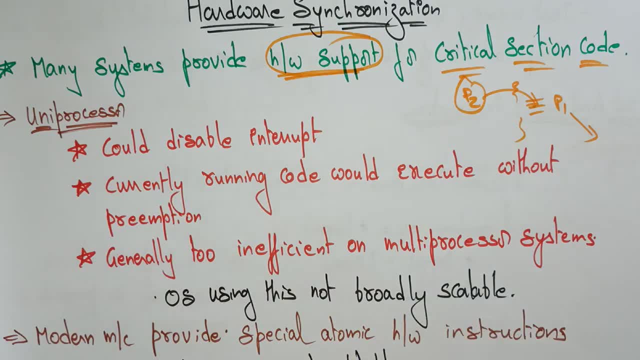 hardware support. So let's take a uniprocessor system. I am taking one of the system as a uniprocessor, So in uniprocessor, how this hardware support will work. So let's take a uniprocessor system. 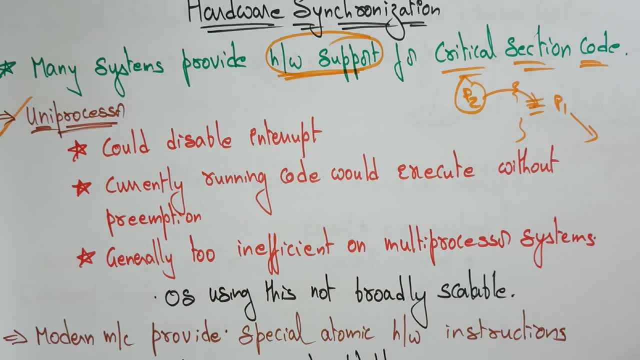 Uniprocessor system is there means my system is having only one processor. So how this one, my system, my laptop or whatever it may be, or whatever the gadget I am using, which is having only uniprocessor. So in that, how, the hardware support is there. So the hard it provides, the uniprocessor provides. 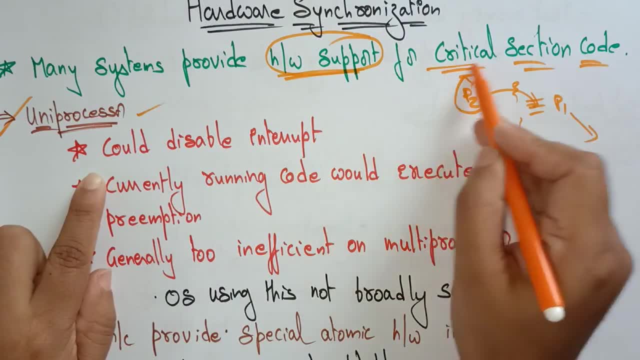 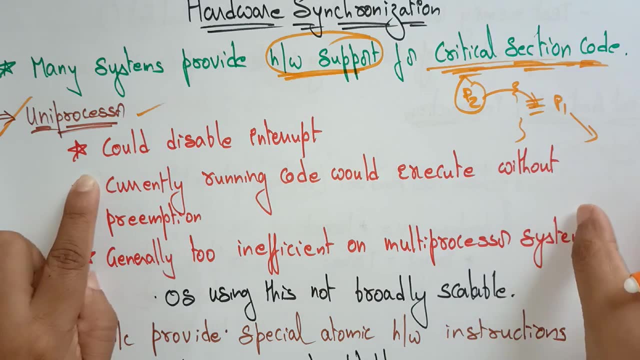 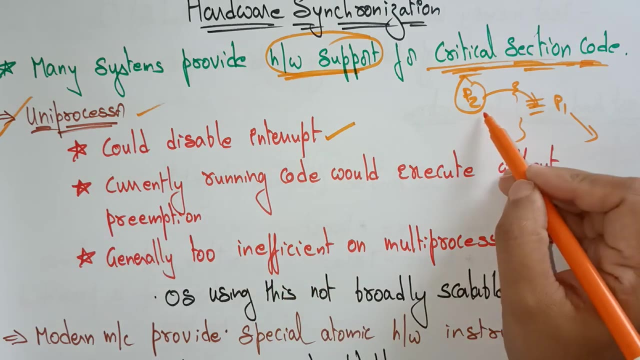 the hardware support for critical section code. I am talking about the critical section code, So how it is going to do hardware support whenever the data is Entered in the critical section code. So first it is doing it could disable the interrupts. whatever the interrupts are there means the P2 is there, P2, P3, P4 or everything on the queue. 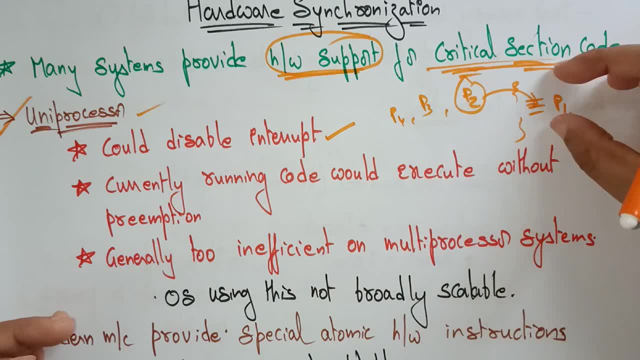 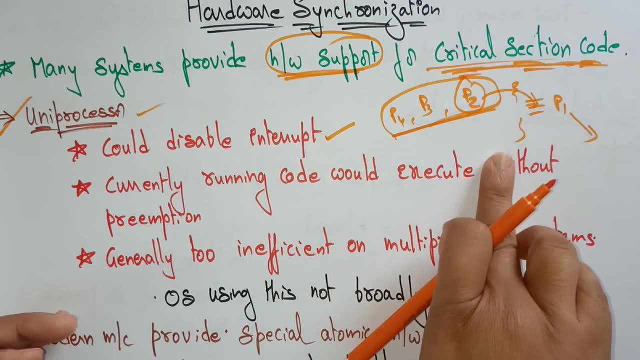 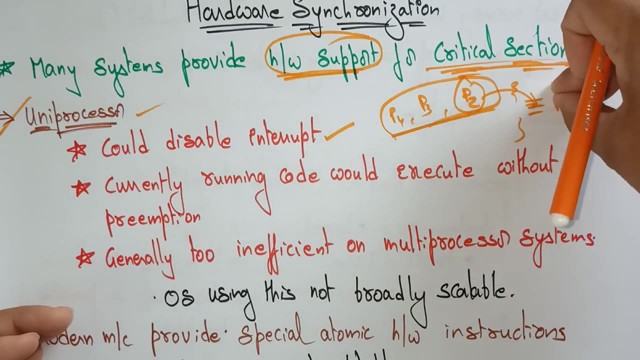 and P1 is executing in this critical section code. So first, what is my hardware support is doing? It is completely disabling all these interrupts. These are interrupts only because whenever my P1 is executing here, the P2 is entering, disturbing it, P3 is disturbing it, P4 is also disturbing it. 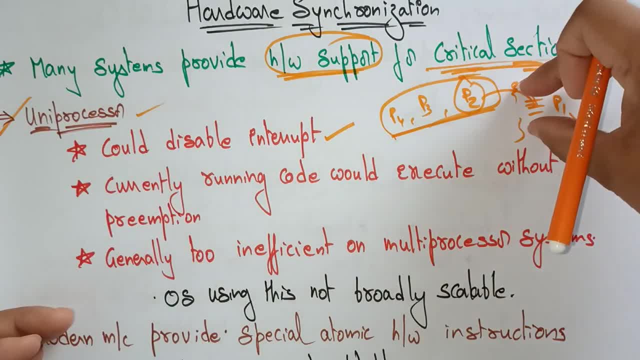 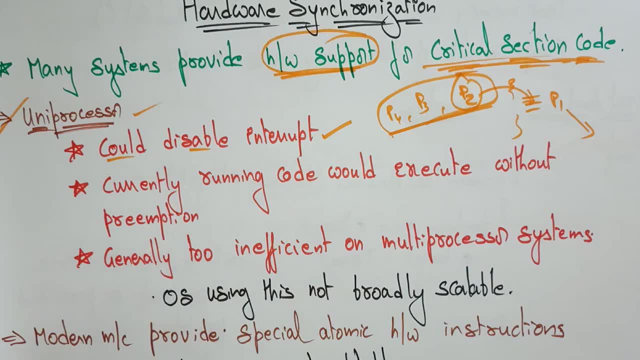 So it is disturbing the processor to stop the instruction and execute my instruction. So to avoid that it's simply disabling the interrupts, My hardware- what is my hardware is doing? It's it disable the interrupt. that currently running code would execute without pre-emission. 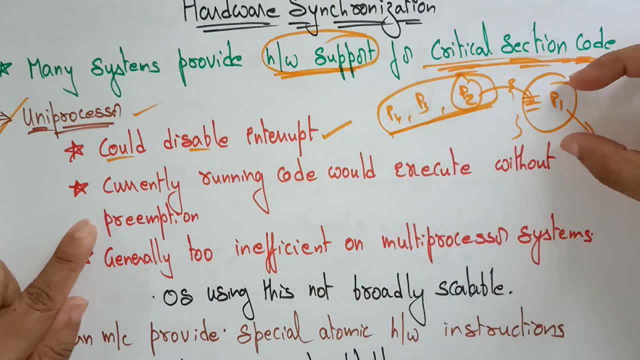 So now my P1. whenever I disable the interrupt, my P1 is calmly currently running. It's execute without pre-emission. Okay, without any Interrupts and without any priority. interrupts will not disturb my process, so it will complete my process. P1 process will be completing its work and exit the critical section whenever it exits. 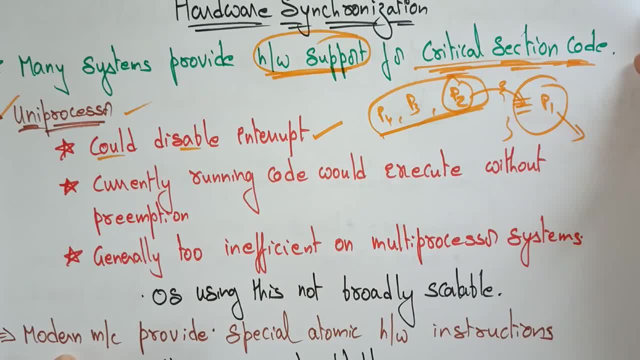 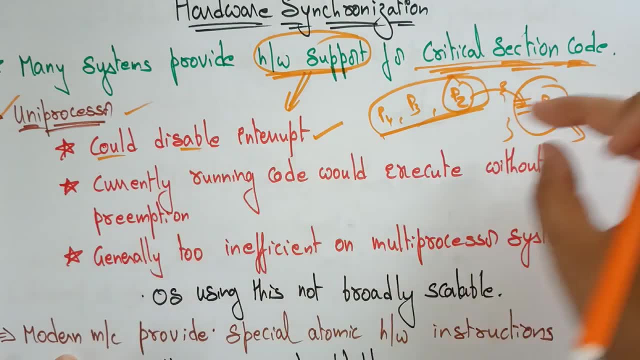 the critical section code, then the another process will enter into the critical section code. So here what my hardware support will do. it first disables the interrupt. whenever it disables the interrupt, the P1 can currently running code would execute without pre-emission. Generally two inefficient. 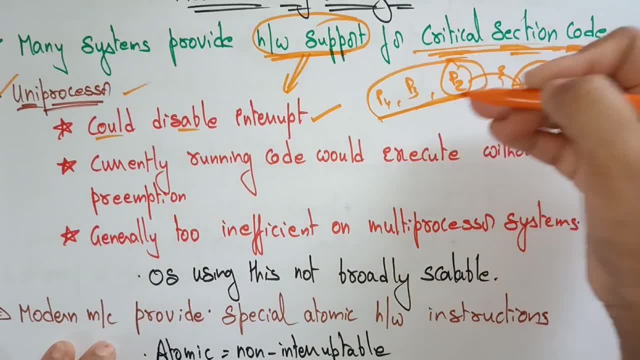 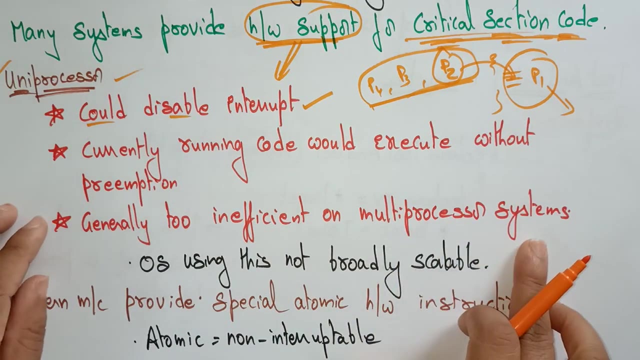 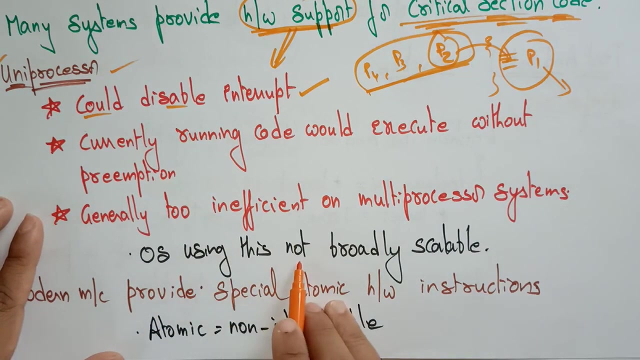 In multiprocessor system. actually this concept, whatever I'm using, the hardware support is there for the critical section just now. I said so generally this is too inefficient on multiprocessor system. so if it is uniprocessor means it's okay, but if you're talking about the multiprocessor system, disabling the interrupts running the current code, it's it's not possible because operating system using this not broadly scalable. 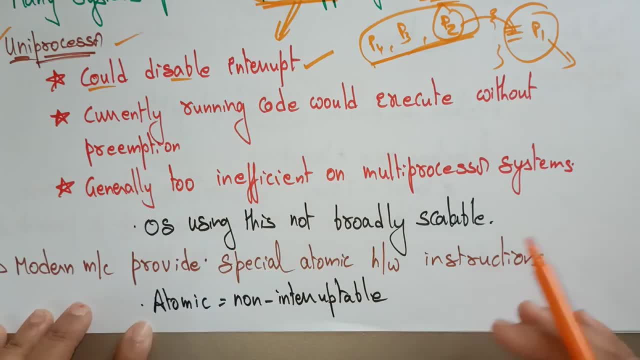 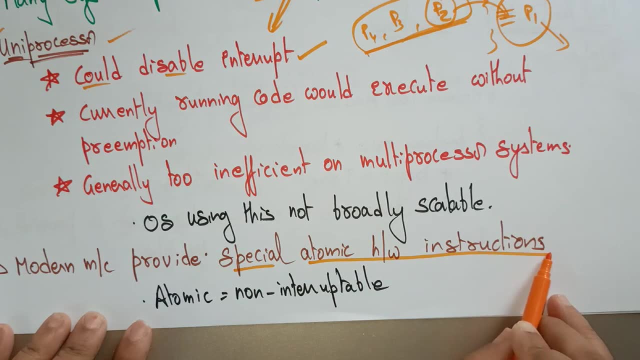 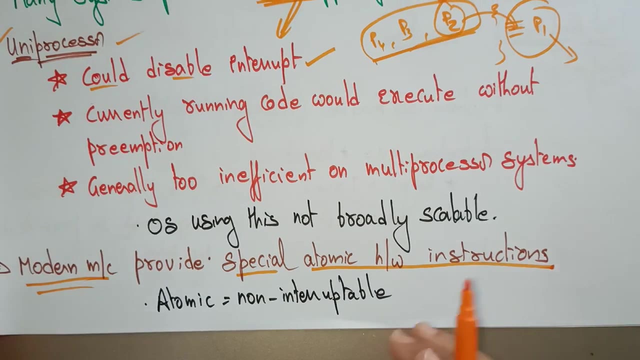 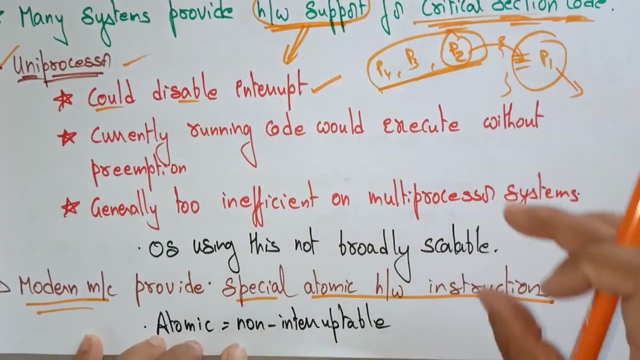 So let's take the modern machine. so Whatever the modern machines we are using, the modern machines provides this special atomic hardware instructions. So here my modern machines, because it is having a multiprocessor systems, will also be there in my modern systems. so it is providing one special atomic hardware instruction. so to to support my hardware, okay, to provide hardware support for critical section, my modern machines provide a special atomic hardware instructions. 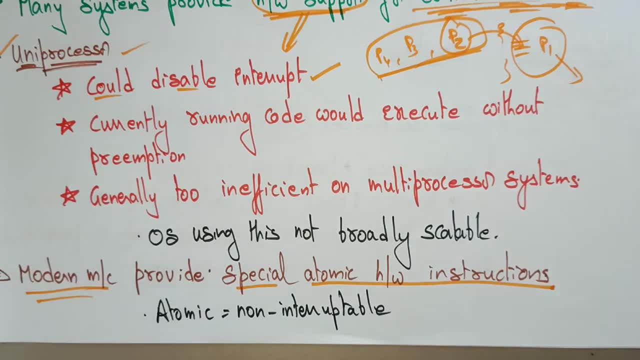 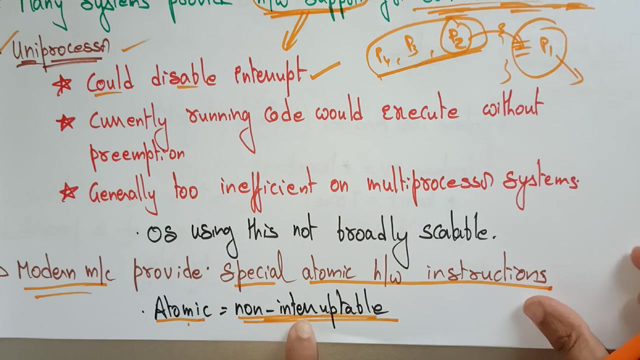 Atomic means That instruction has to be executed without interrupts. my, my instruction has to be my process P1 has to be executed without interrupt. So that is the meaning of atomic. atomic means non interruptable. it is not interrupting anyone. so these modern machines provides a special atomic hardware instruction that is atomic. so we call it as a non interruptable and also it use it, do some in. 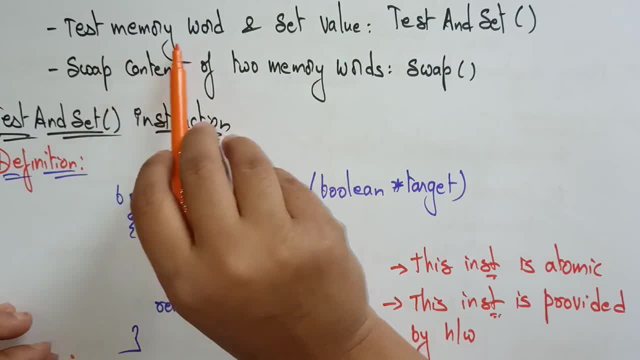 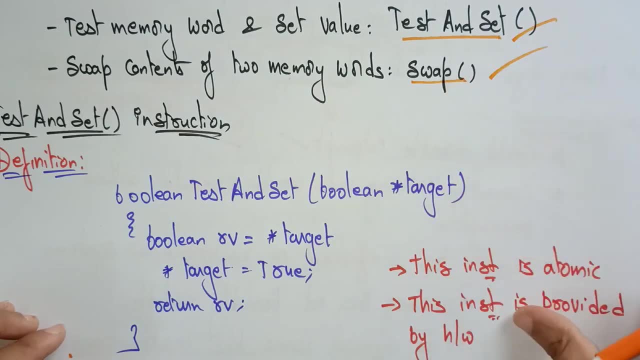 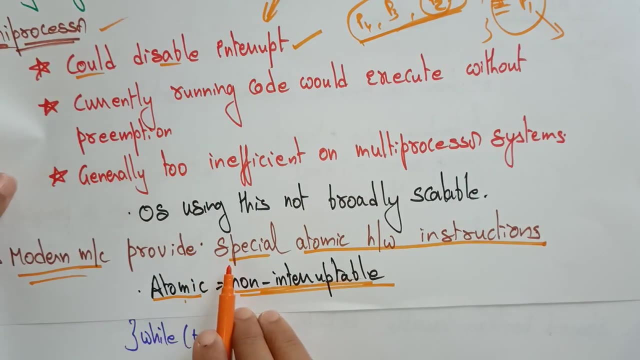 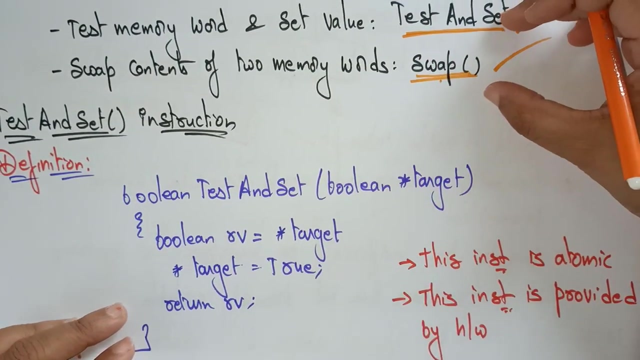 Coding. So I'm using a test set, test memory word, and sit right. It's 10 set and the content of two memory words. that. so we, the help of these, These functions, with the help of these functions, My model machines provides okay, especially atomic hardware instructions. so these are my hardware instructions. 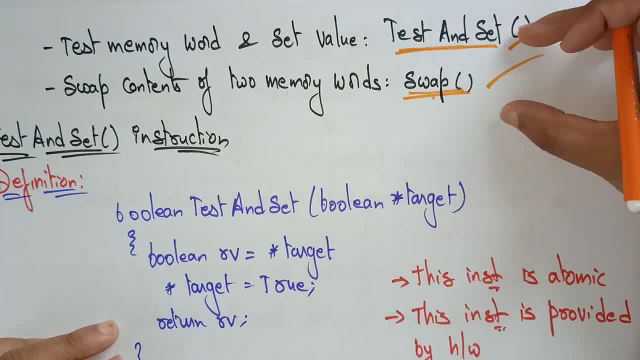 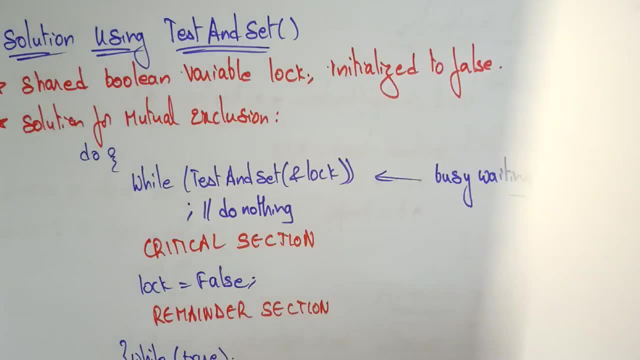 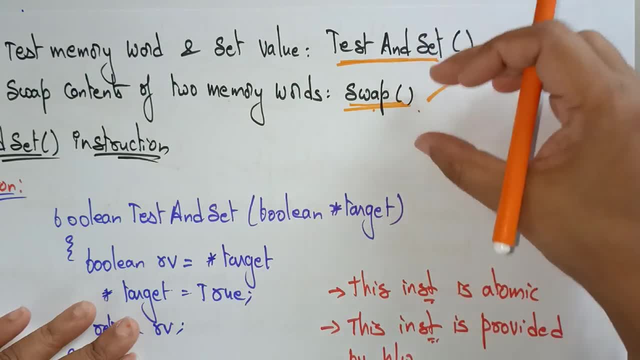 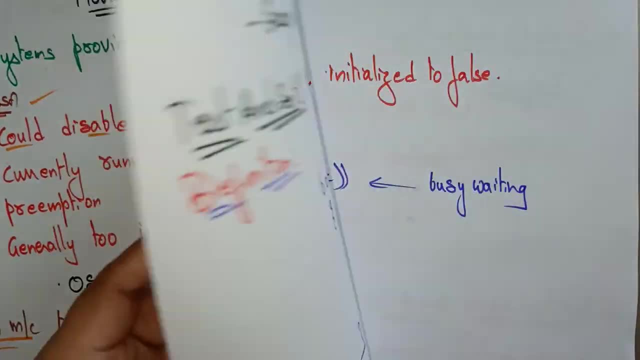 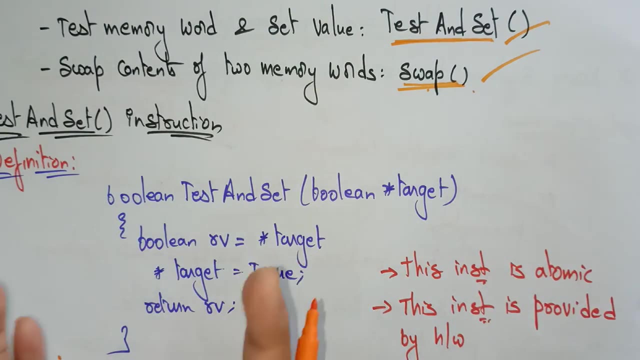 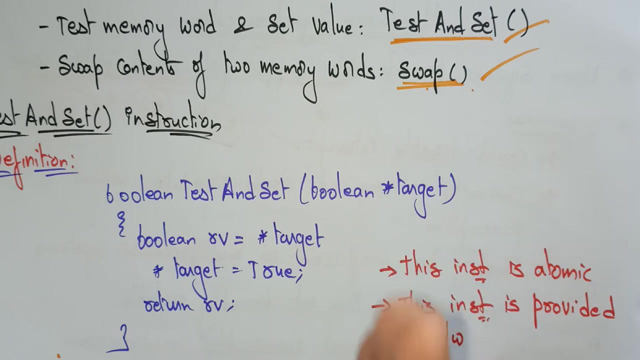 is these: test and set and swap. so these are the two hardware instructions. these are the two atomic hardware instructions. okay, so which are support for the critical section code? do you understand what exactly the hardware synchronization is? if one operation has to be executed, my critical section code has to be executed without interrupts means my atomic instruction. that is my atomic. 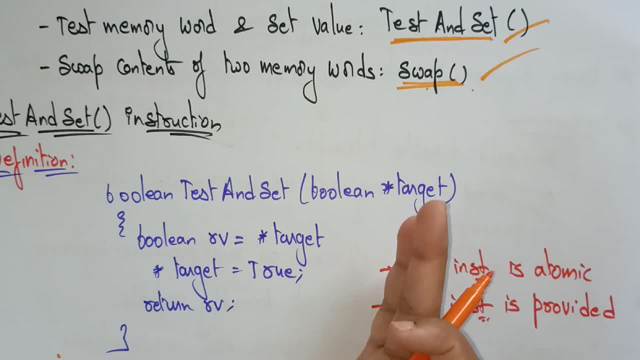 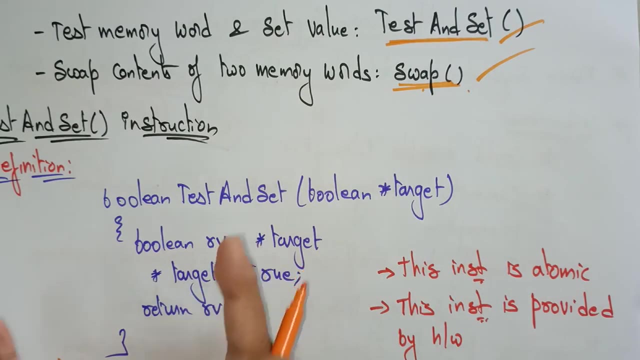 instruction that is non-interruptible. instruction has to be executed without any disturbance means there should be hardware support is also required. so for hardware support it should be synchronized with the critical section. how it is going to be synchronized? so, with the help of some atomic hardware instructions. so what are those hardware instructions? test and set and swap, let it, let's. 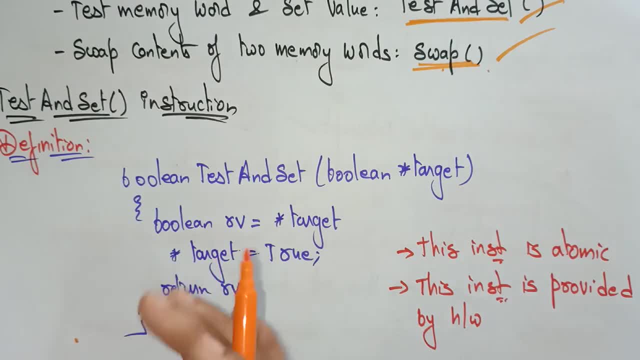 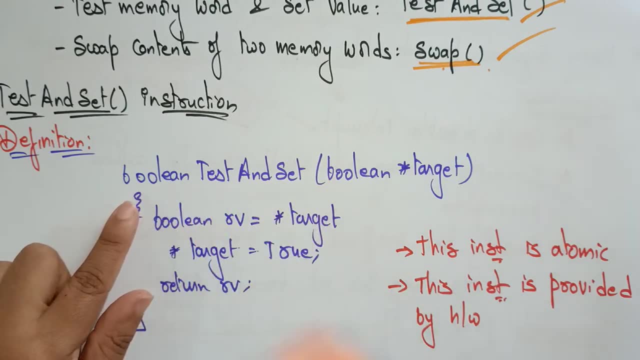 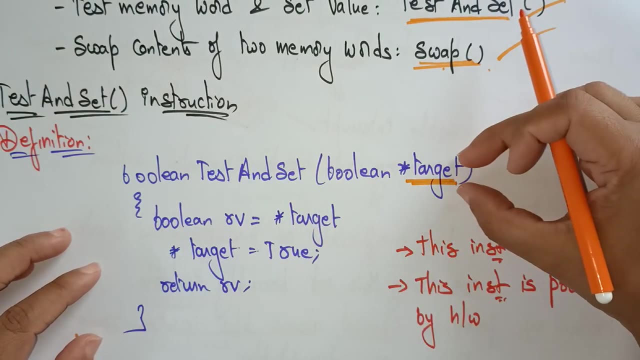 look on this test and set, actually my test and set instruction is defined as boolean value. okay, either zero or one. so test and set test zero and set one boolean. my, it's my target, okay, my, my process. that has to be executed. so i am assigning the target, a pointer target, to rv value. so whenever my target pointer- 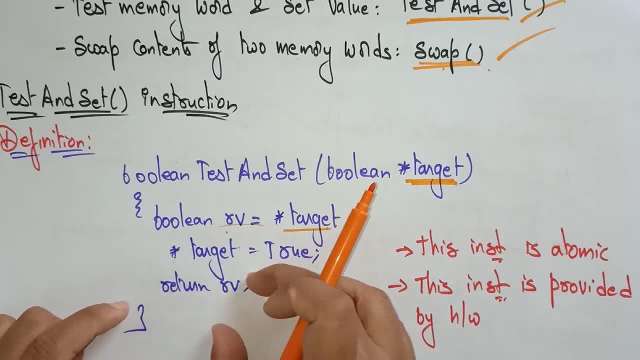 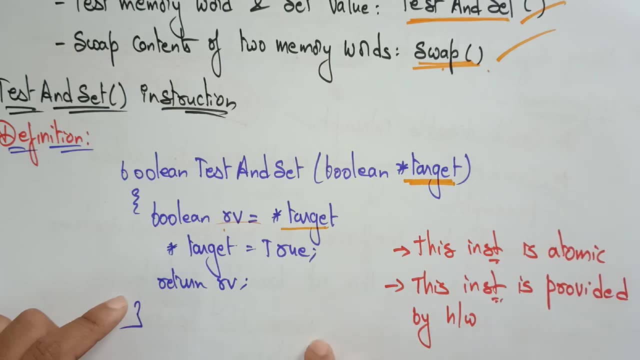 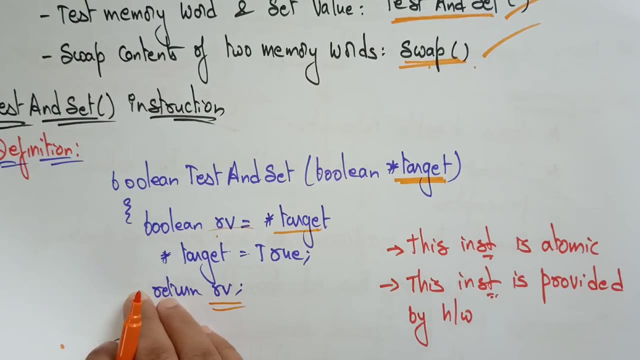 is true? okay, i have to return that. i have to enter into the critical section that has to be executed. so this is my atomic value. so this instruction is atomic and this instruction is provided by the hardware. so this complete in this instruction now will be provided with the hardware. now this has to be synchronized. how i 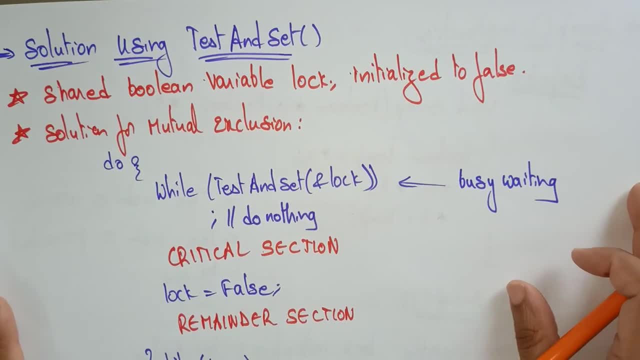 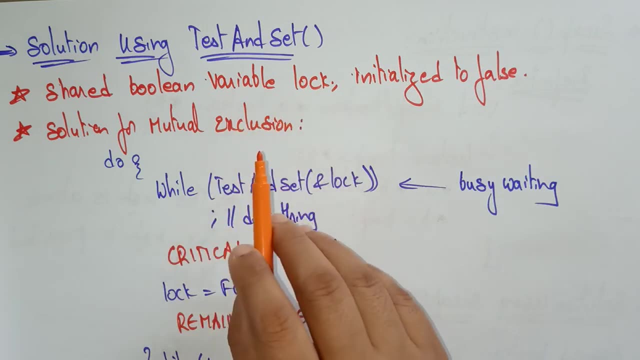 am going to be synchronized. the solution for this test and set is shared boolean variables. uh, are there, because, uh, the boolean variables has to be shared by all the processor. uh, the different process wants to enter into the critical section. the shared boolean variables are there, so i am taking it as a lock. so whenever the variable is locked, it is initialized to false means here one. 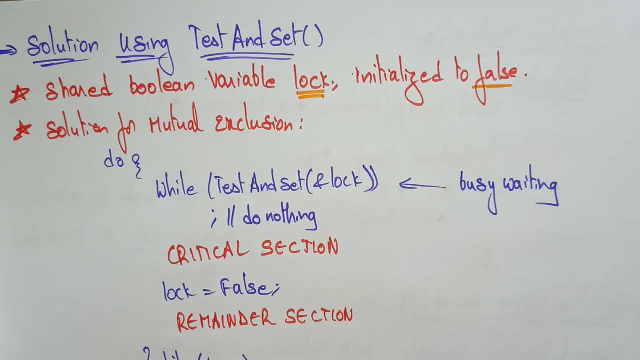 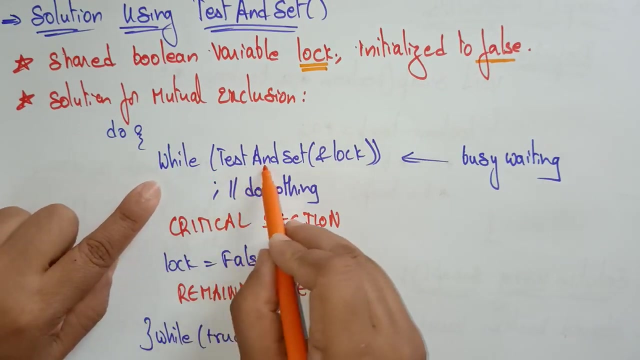 of uh process is enter into the critical section. that is an atomic instruction. enter into the critical section so it should be locked and it is initialized to false so that the other instructions will not enter into this section. so this solution for the mutual exclusion is: do so first. why the test and set? this is my hardware instruction. 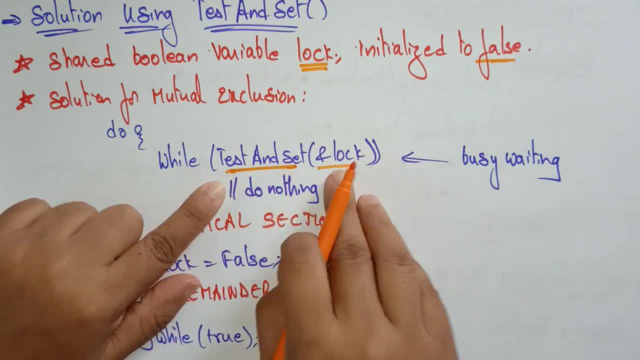 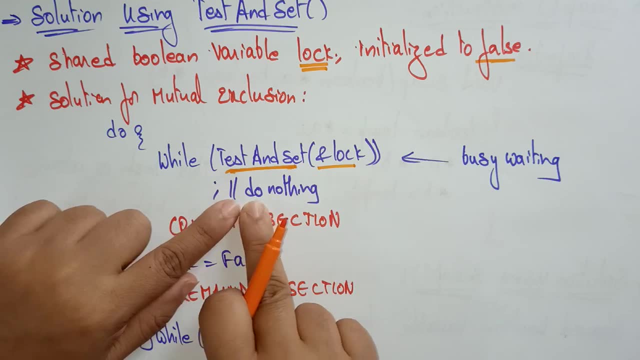 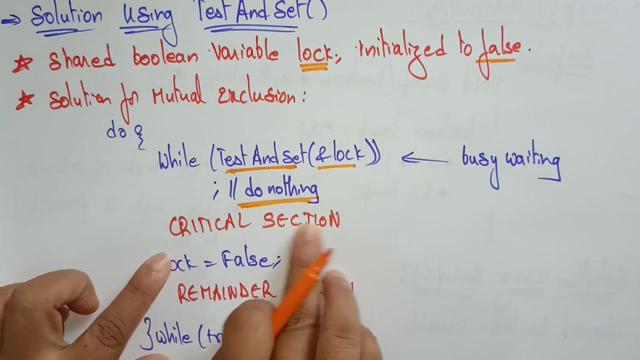 the test and set is lock whenever the lock is there. whenever it is lock is there, it is a busy waiting. okay, it is busy waiting. so means something is entered into the critical section. whenever something is entered into this critical section, the test and set will not do anything. okay, it's. 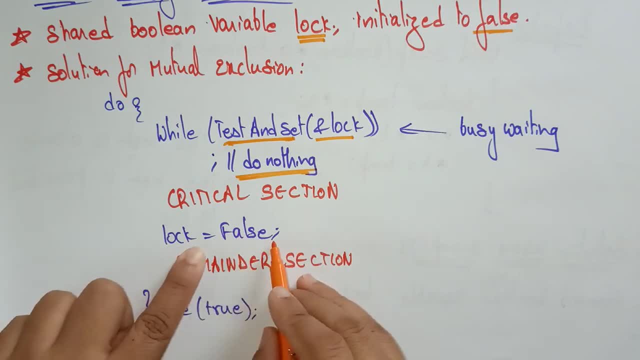 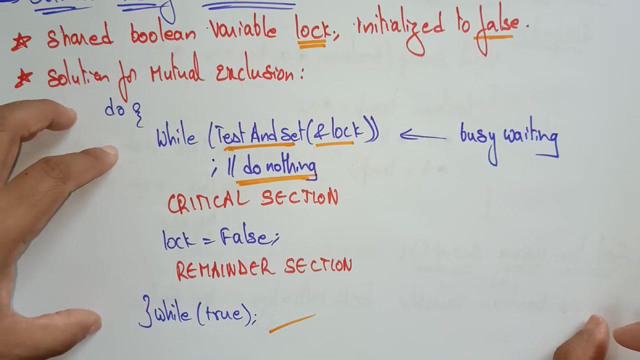 said: enter into the critical section, okay, and lock falls. whenever the critical section is over, the operation is over, it releases the lock and remainder of the section it enter. it do what it works with the reminder section. okay, and while true, so this is a solution for the uh test and 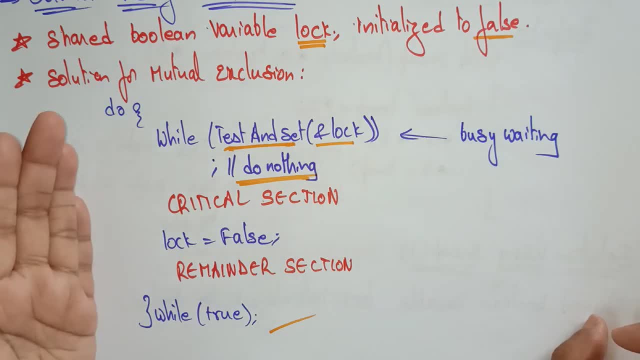 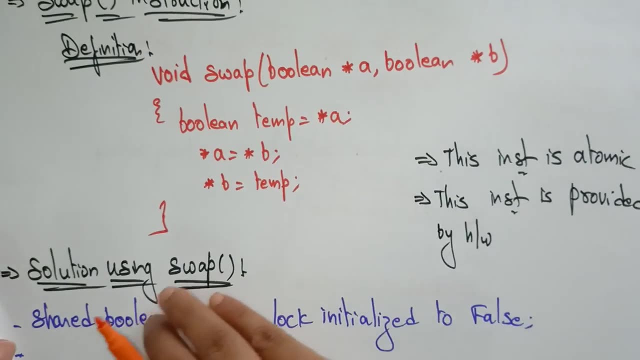 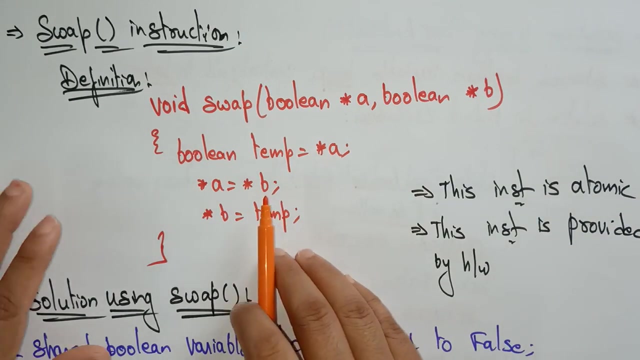 set hardware instructions for uh synchronization, to maintain the synchronization. so this is the concept you have to be followed. so let's take the another instruction, that is a swap instruction. i said that one another hardware instruction is a swap instruction, so what this swap instruction will do? so this is my basic definition of this wrapper void swap boolean. 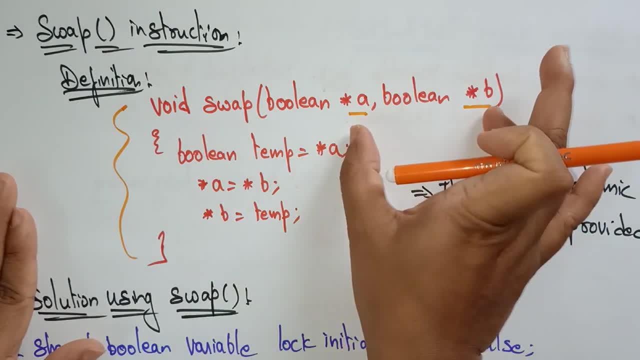 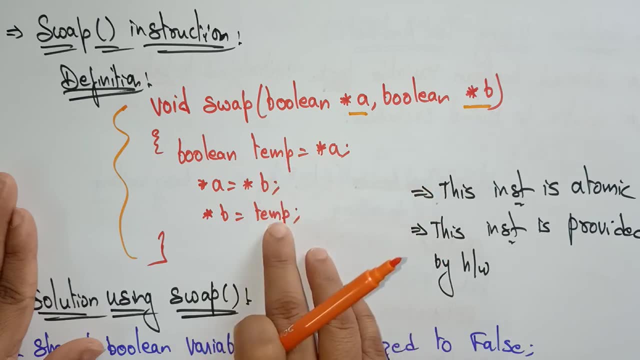 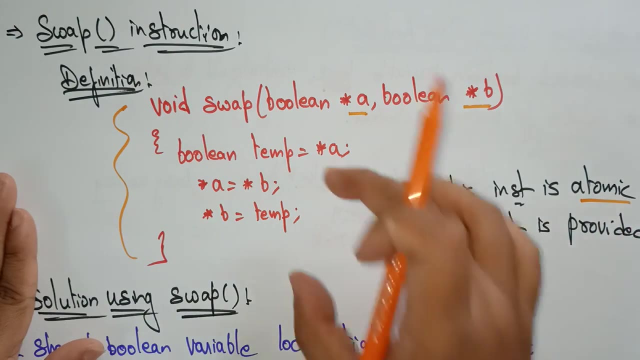 values. i'm taking two boolean values, so now i am going, i'm doing the swapping. so a has to be pointed to the temp variable. now my temp contains a and that a name should be moved to the b. okay, so this is also my atomic instruction. so this instruction is provided by hardware. 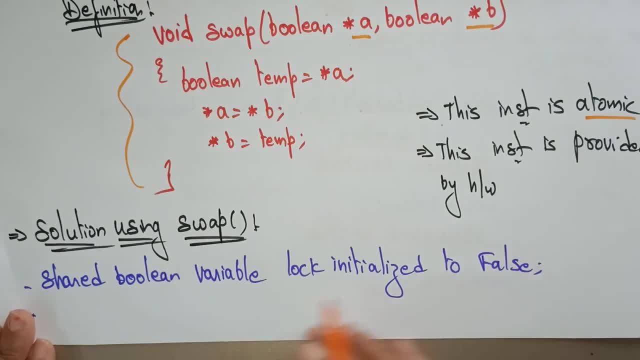 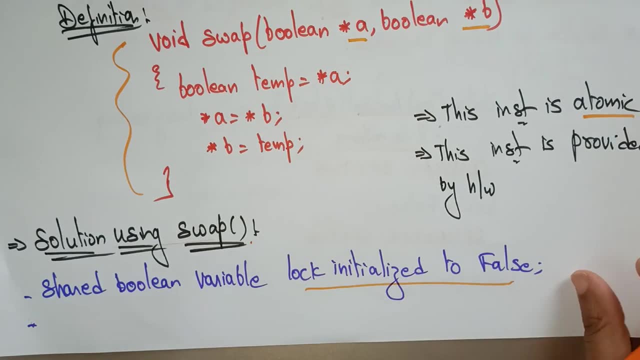 these instructions will be provided by hardware. now let's have a look. solution using swap: the shared boolean variables lock initialized it to false, so just like a uh boolean value is stated now, this examples is possessive because it is not tied to theThere are no stitches if box randomly selected, universal being locked means that sẽ ch задачure嗯, and. 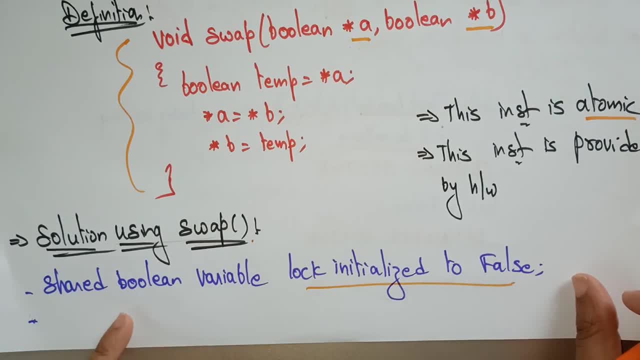 these instructions will be provided by hardware. now let's have a look. solution using swap: the share boolean variable lock initialized it to fall, so just like a. uh, whatever the з the test and said we had seen that. so here also for the swap also you have to do shared boolean.